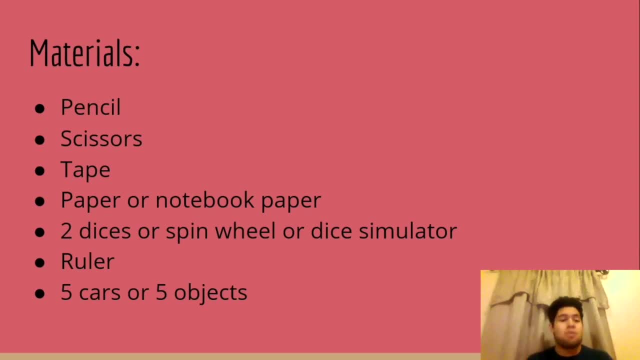 a link down below the comments. if you guys want to try it out, Alright, and you're going to need a ruler And five cars, You see: Alright. so if you don't have five cars, you can just use any five other objects: Five LEGO's, five cubes- whatever you have at home works, Alright. 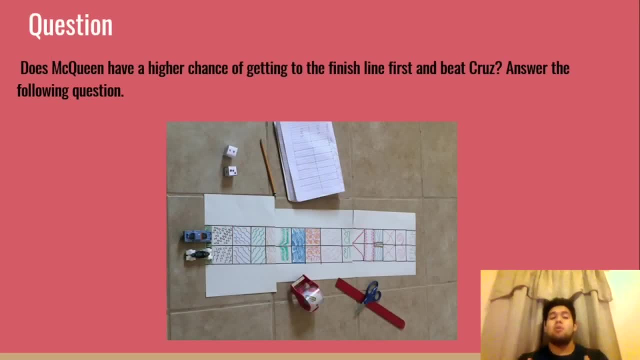 so the question you're trying to answer- now I can use a Н rap, If you want you can pick- is this: McQueen, have a higher chance of getting to the finish line first and be cruise. you'll be able to come up with an answer after you answer the following. 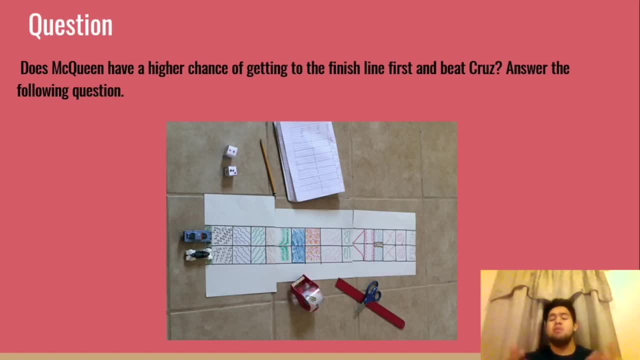 questions. by the way, as you can see in the picture, this is the design of the racetrack that I made. this is just an example what you could do, but you can be as creative as you want and creating your racetrack it is up to you. just have. 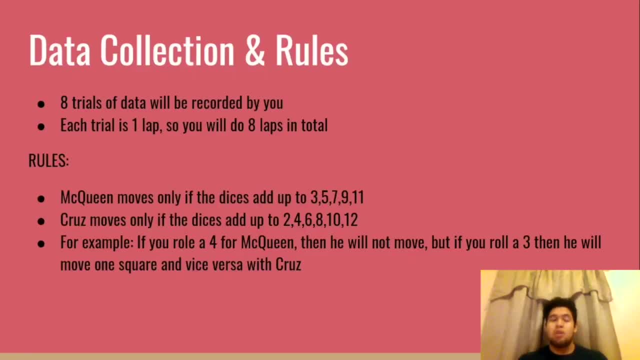 fun guys. alright. so data collection and rules. eight trials of data will be recorded by you. each trial is one lap and you will do eight laps in total. now rules: McQueen only moves if the dice is add up to three, five, seven, nine, eleven. Cruz moves only if the dice is add up to two, four, six, eight, twelve, for example, if 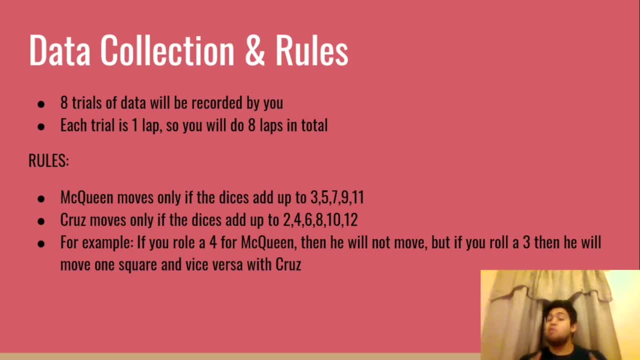 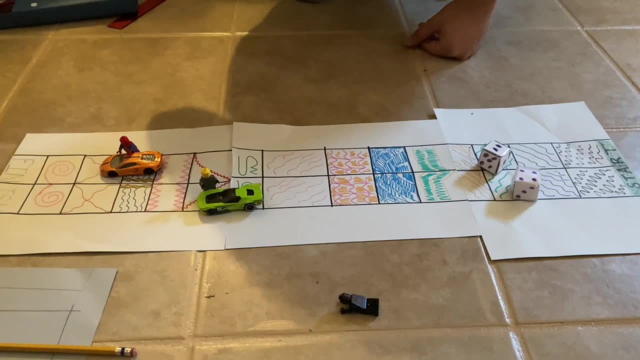 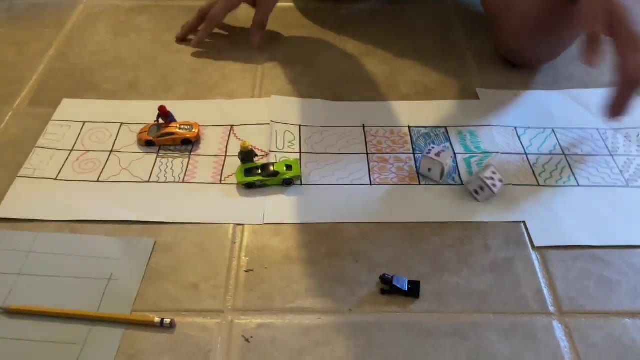 you roll four for McQueen, then he will not move, but if you roll three, then he will move one square, and vice versa with. now would you math enthusiast? so before starting the recording, my brother and I have been playing the game, so now it's my turn. all right, so I got a six and a one six. 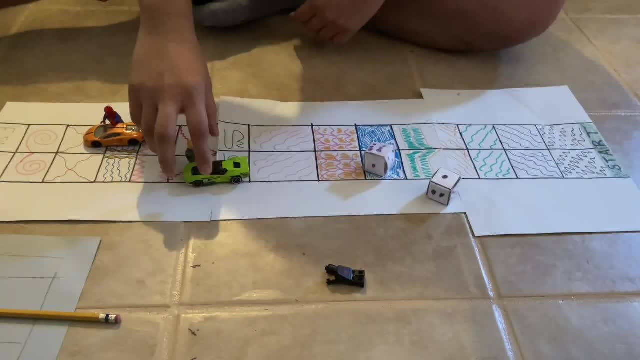 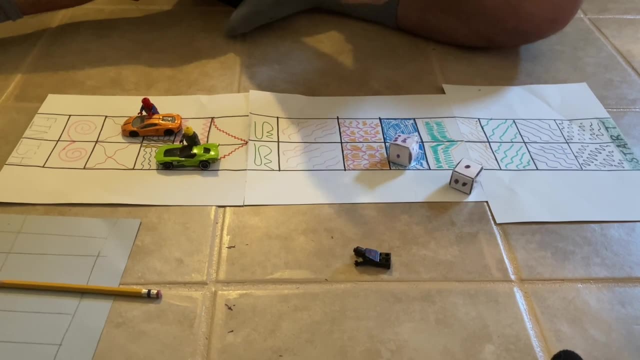 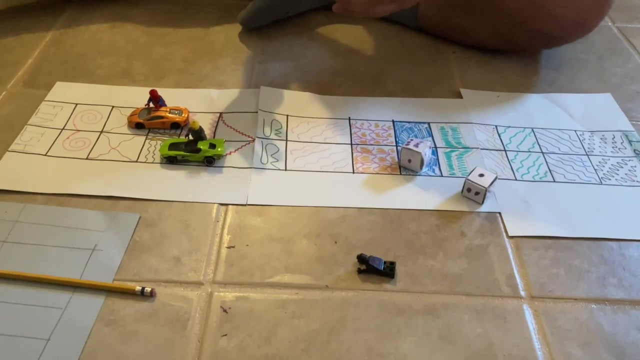 plus one equals seven and I will move one square up. all right, I can only move up if I roll a three, five, seven, nine, eleven. I am pretending to be McQueen, my brother's pretending to be Cruz. so if my brother rolls a 2, 4, 6, 8, 10, he can move 1. 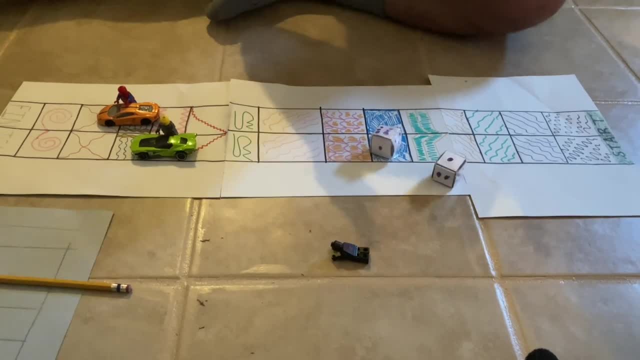 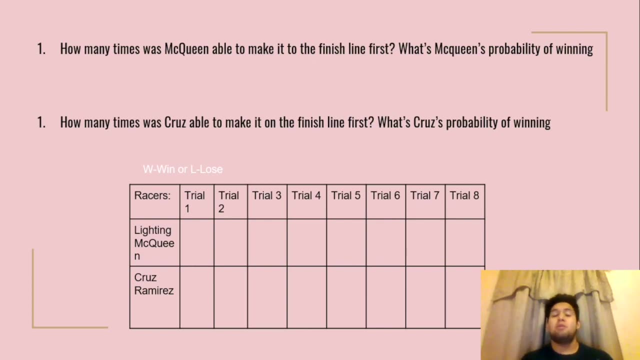 square Ab Davidson, like 6, 2, 5 and I will move one square up, all right. so now that I'm gone, it's my brother投 continuer right. so now that we have a better idea of how the security is going to work out, we can answer the following questions.